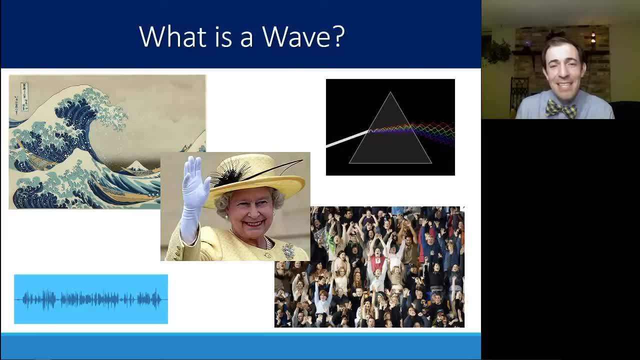 not so much. I want to start by giving some examples of these waves, starting with one that is really based on simple harmonic motion using a pendulum and changing the length of one pendulum relative to the one next to it. so the period changes and the result. 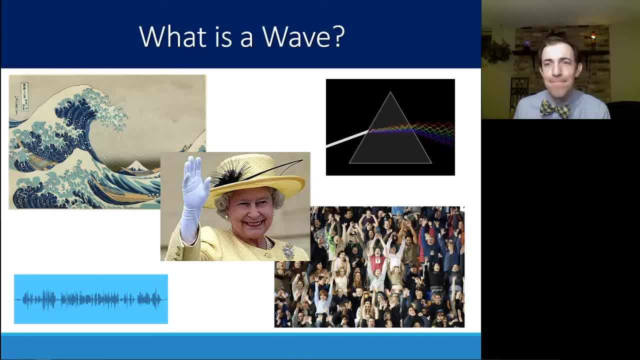 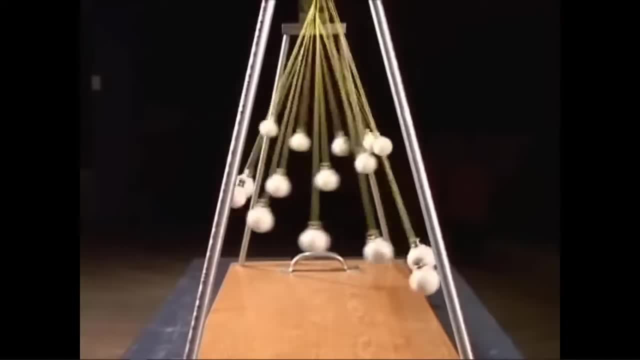 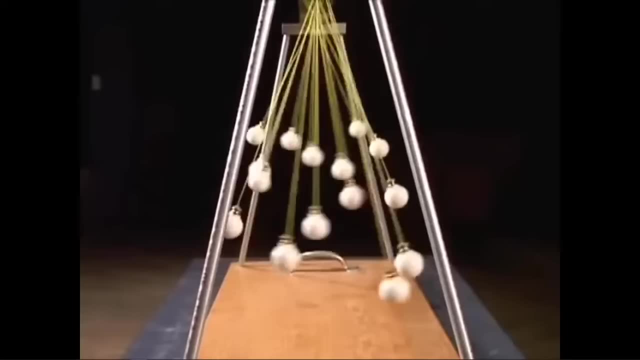 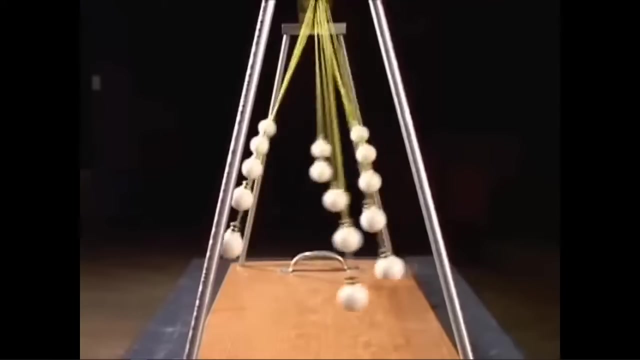 is some pretty cool waveform shapes that are formed. So we're going to use the same formula with a set of basic twiceklich waves. The first wave is a set of two different frames. The second wave is a set of two different types of waves. 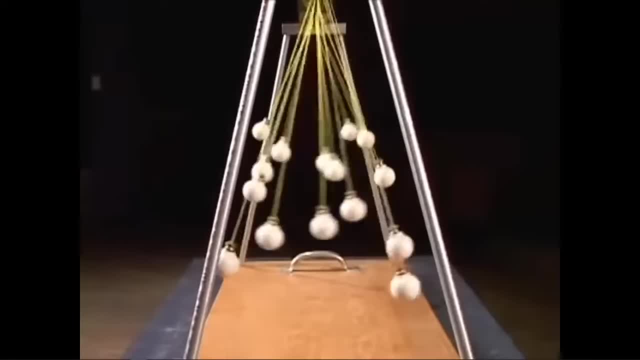 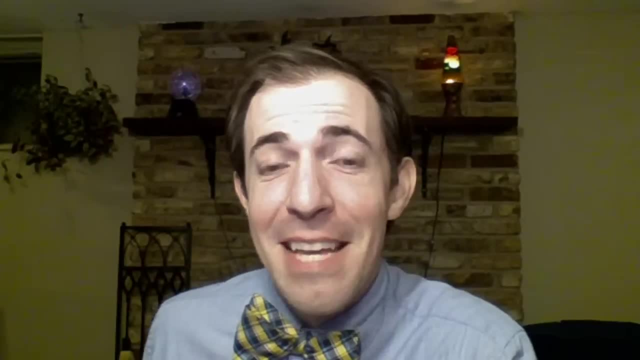 And then the first wave is a set of two different types of waves. The third is a set of two different types of waves. So the first wave is a set of two different types of waves. If I would have let that play out, it would have actually continued along and kind of reversed. 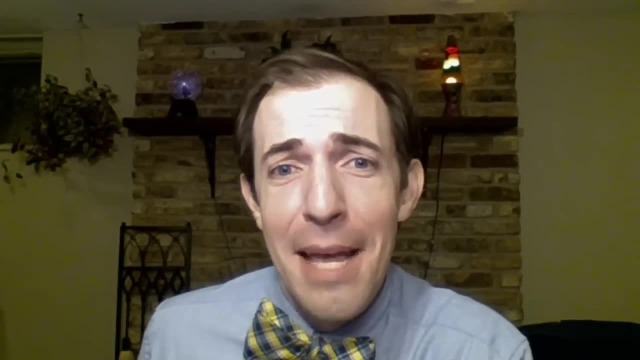 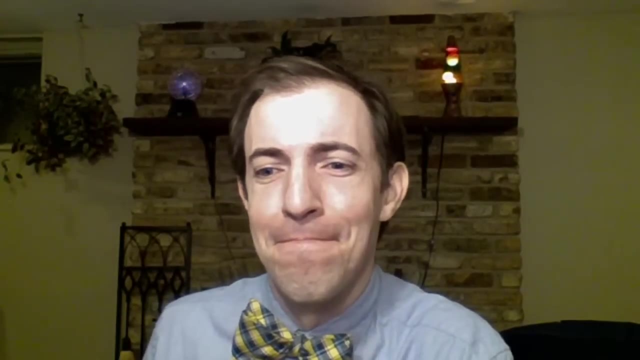 itself to end up sitting in this comfortable space up back, in one single line. the next example of a wave is one that some of you have maybe experienced before, and that's a wave made out of people. it's a stadium wave, a new world record for. 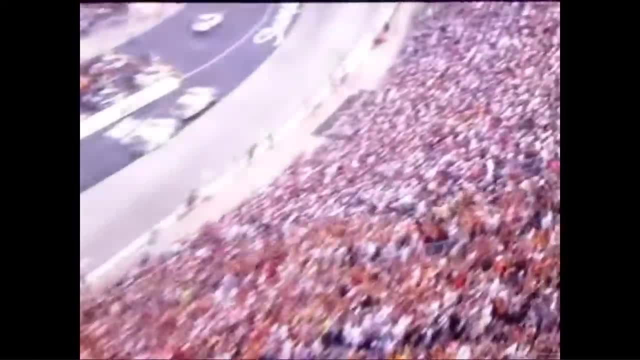 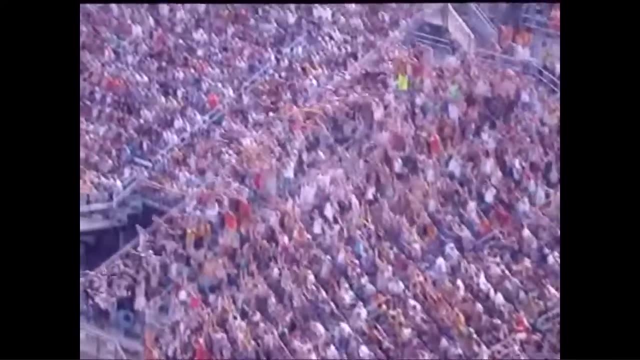 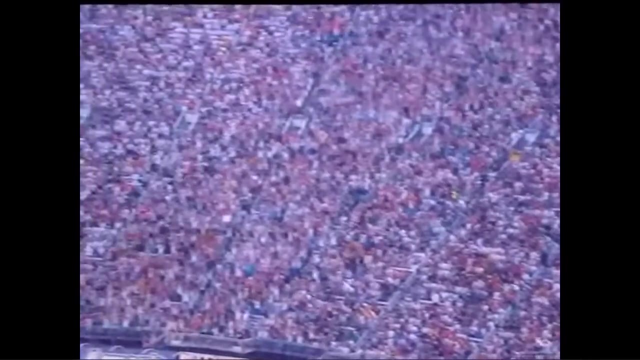 the wave attempt. can they do it? 168 000 they are here from the guinness book of world records to certify the record if they can make it all the way around. yes, folks, just another sellout crowd here at the world's fastest half mile in bristol, tennessee. the next example is a really important 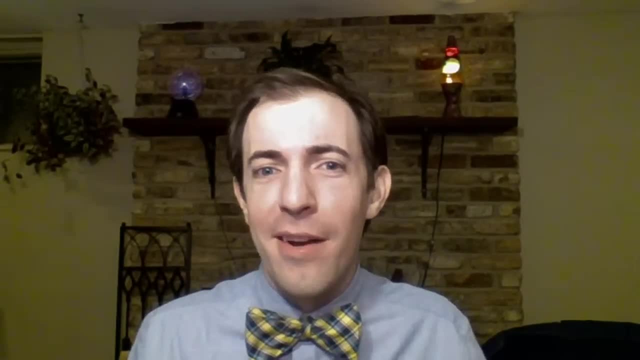 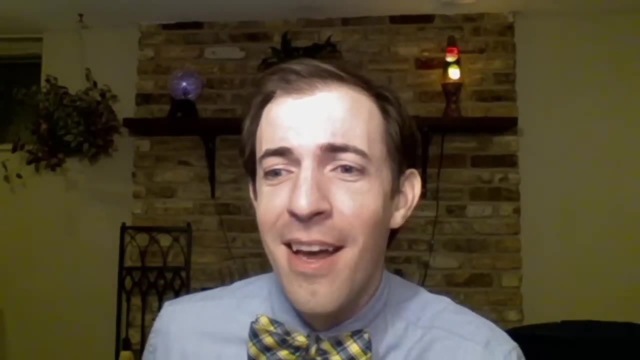 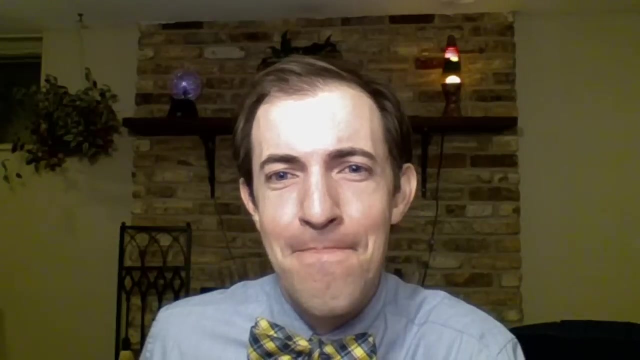 one. when we talk about physical waves, and that's a wave made out of water, it's your classic water wave. uh, the video i want to show you here is the largest water wave. it's a tsunami just off the coast of japan. this is what the tsunami that hit about a decade ago, what it looked like, um, when it. 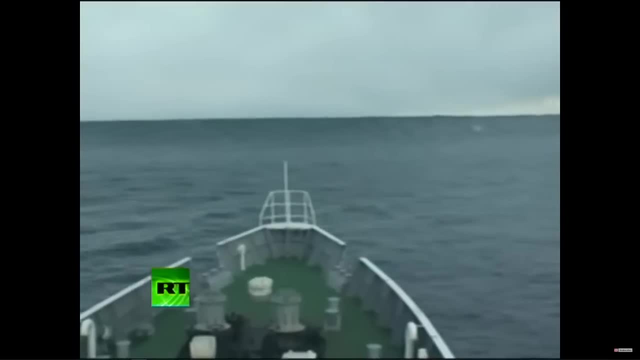 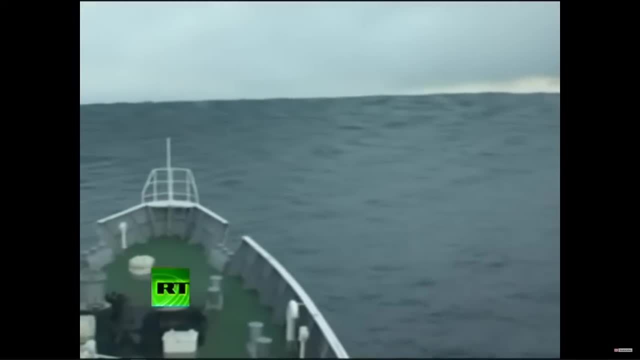 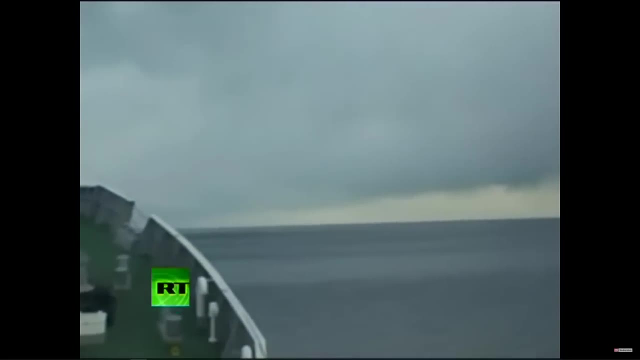 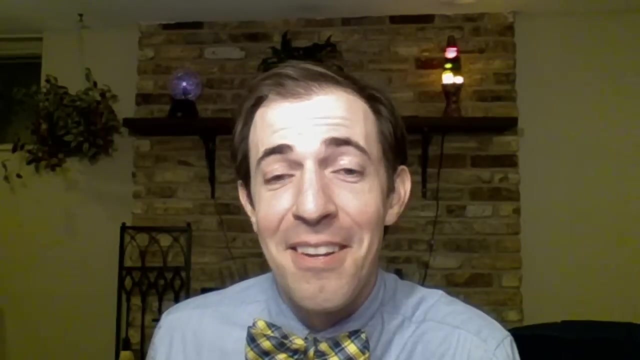 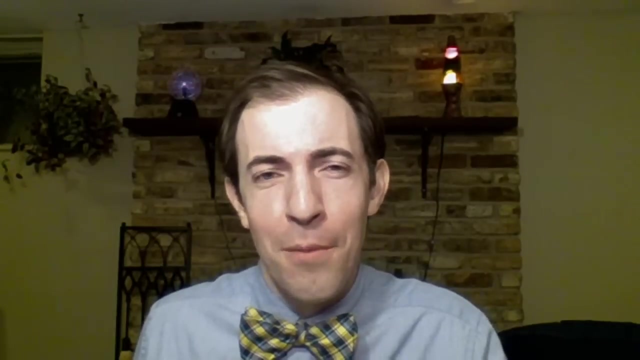 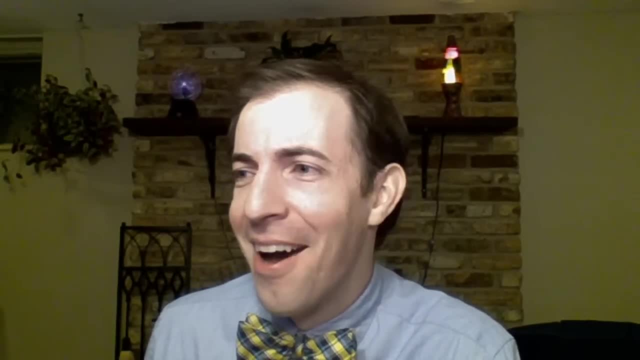 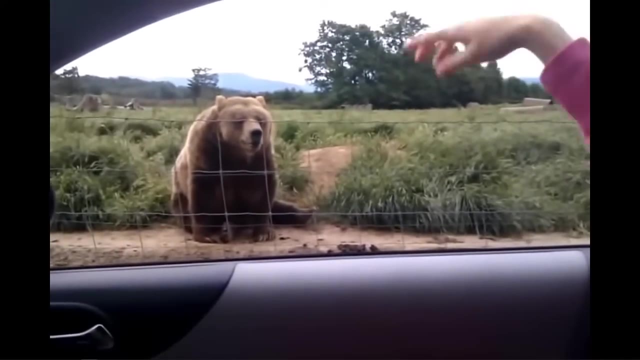 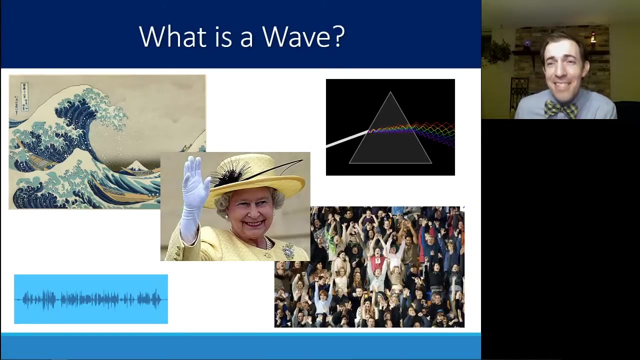 to the next uh. and then i want to end off with one uh example just for fun. and then i want to end off with one uh example just for fun, All right. so all of those are examples of different types of waves, and with the exception. 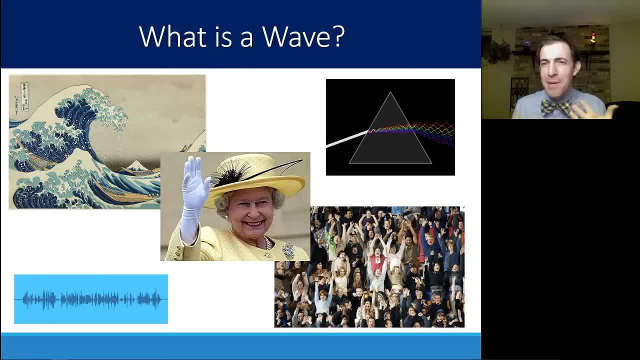 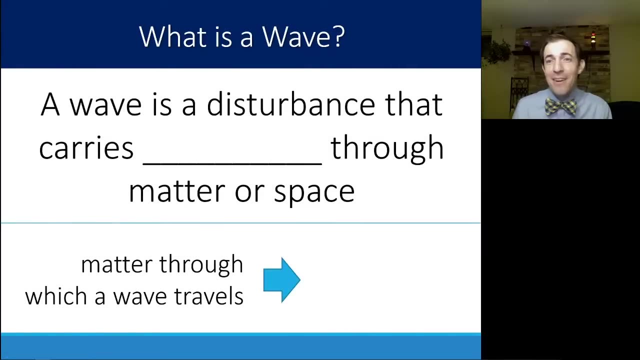 of maybe that last one. all of them can be defined using the same terminology and potentially even the same numerical quantities as the waves that we're going to be talking about in this class today and beyond. All right, so what is a wave? Our definition of a wave is going to be: a wave is a disturbance that carries energy. 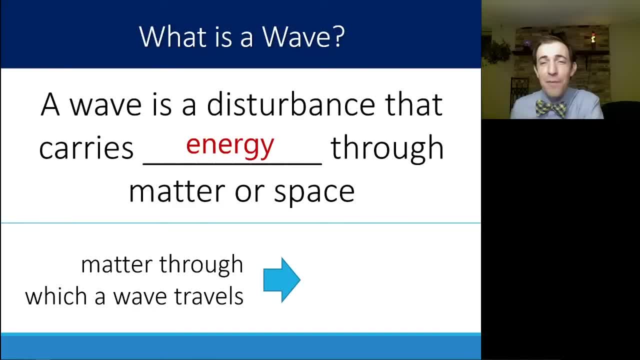 through matter or space. It's basically just a way of transporting energy from one place to the next, whether that's light or sound, or some mechanical wave like the tsunami carrying energy through water. All of these waves- with the exception of light, which we'll talk about- require matter. 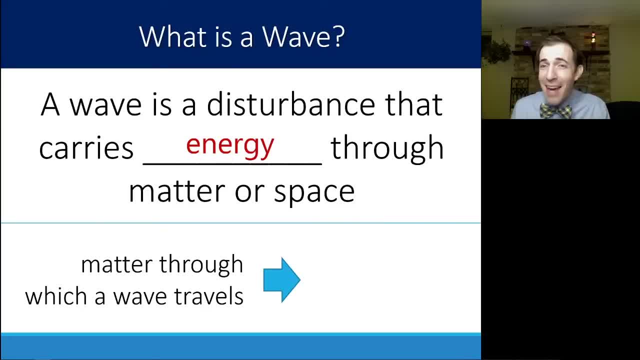 to travel, for that wave to travel through. That matter has a name which you may remember from a previous class. that is the medium that the wave is traveling through. Right now, my voice is making it into the microphone through that distance, through the 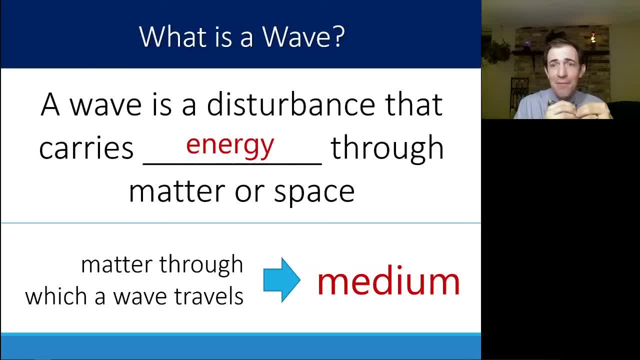 medium of air that it's vibrating the different air molecules to allow it to travel. Sound requires a medium in order to travel. There is no sound in space because there is a vacuum. There's no air in space. There's no air in the deep outer space. 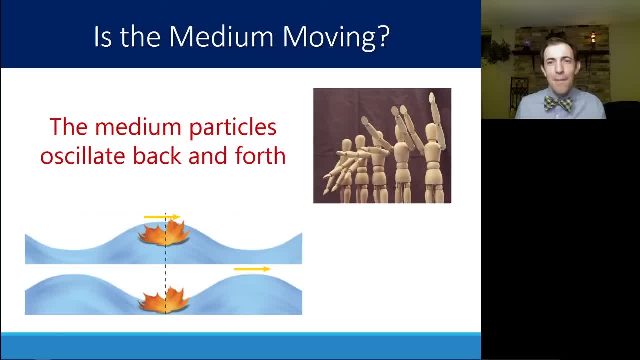 So this idea of a medium is really important, but it's also important to know how that medium is moving. The medium particles, they oscillate back and forth. So just like you're seeing there the actual text oscillating back and forth, the letters, 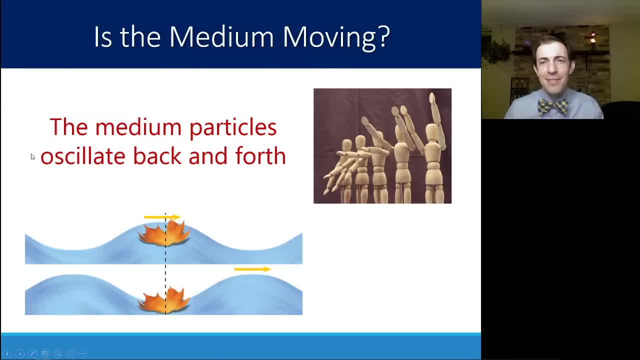 are going up and down, but the wave is traveling sideways. So those particles, they do vibrate, but they don't necessarily move with the wave. They don't move with the wave, They don't move with the wave at all. Think of it like a leaf that flows up and down, or that boat flowing up and down on the tsunami. 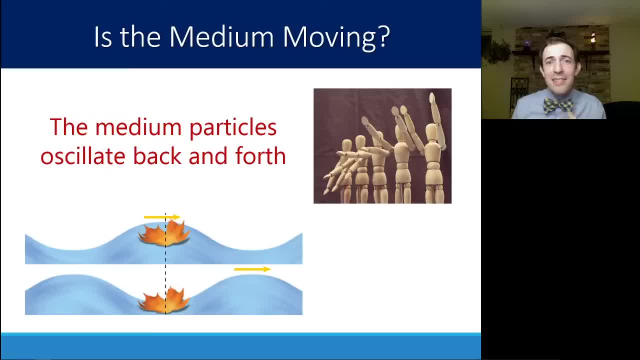 The boat didn't surf the tsunami, It didn't travel the whole way. And the same thing is true with the different particles, the different molecules of water along the way. in that medium, In a stadium wave, the medium is the people, The people. they go up and down but they're not running with the wave. 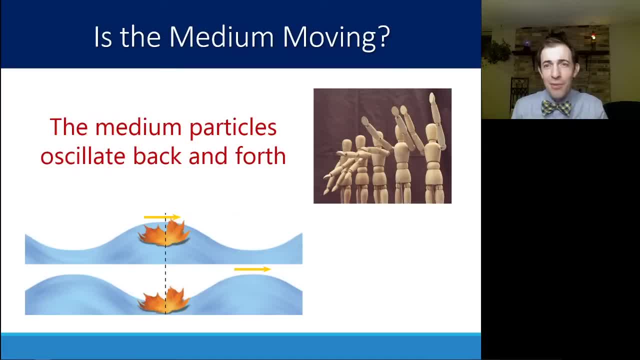 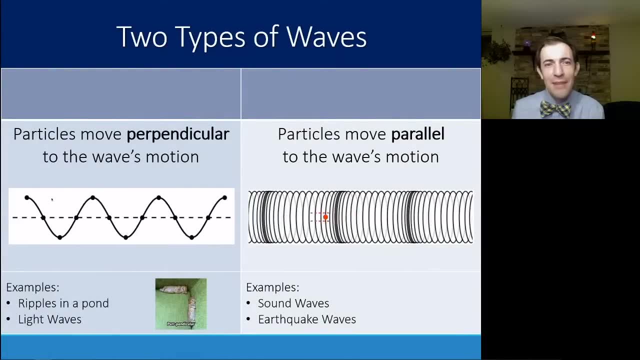 The wave can travel without the medium needing to travel with that wave, So they're vibrating back and forth, not traveling with the wave itself. There are two main types of waves that you need to be familiar with in our categorization of these waves. 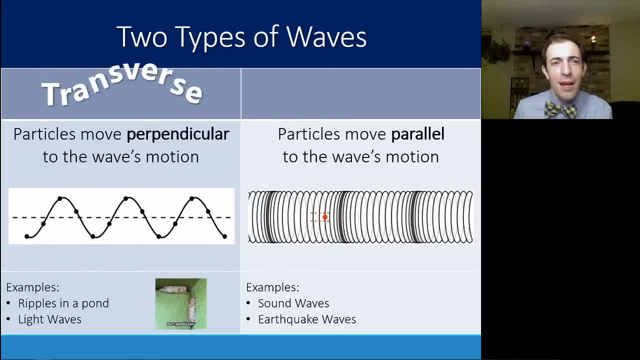 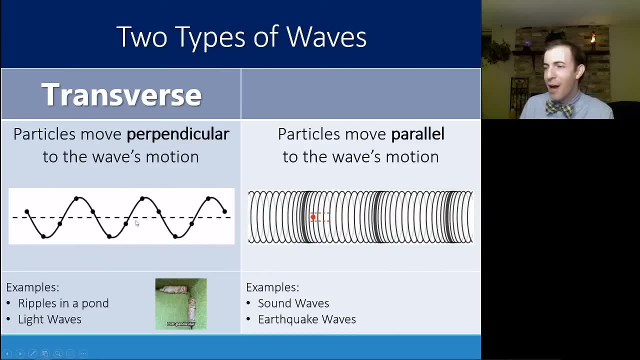 The first is known as a transverse wave. A transverse wave is when particles move perpendicular to the wave's motion. Here is an animation of a transverse wave. Now I want you to take a note of what one of these dots is doing. 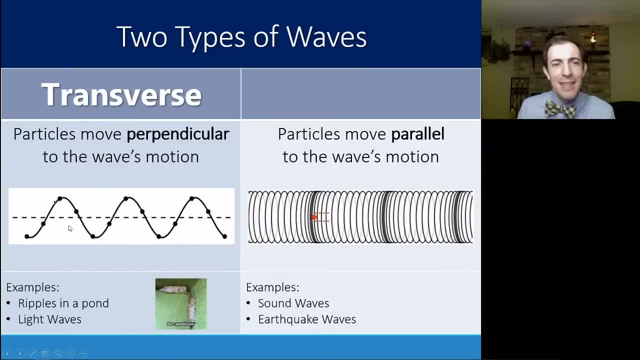 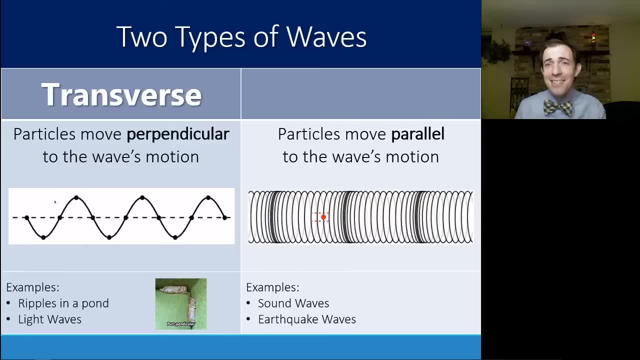 Clearly the wave is moving to the right, but these dots individually are just moving up and down in their designated spot, Kind of like the stadium wave people going up and down while the wave moves along. These particles are moving perpendicular to the wave's motion. 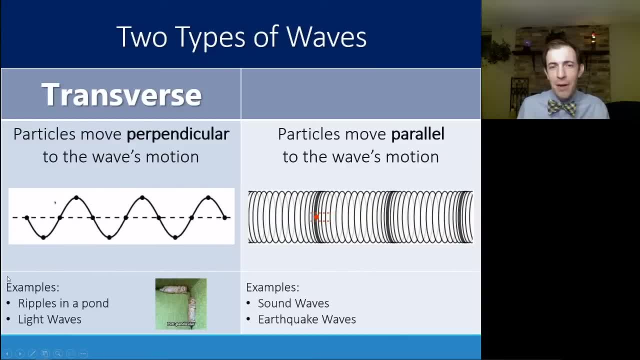 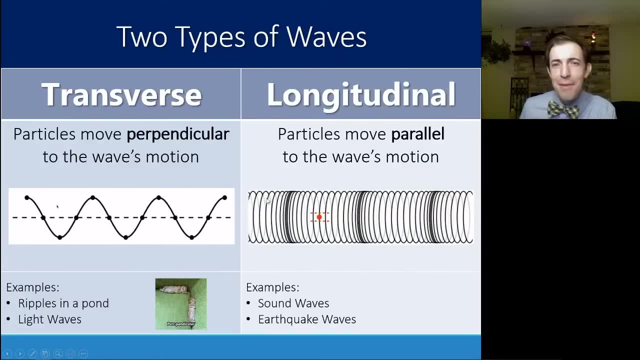 So examples of this are like ripples in a pond or light waves: They are always perpendicular. The other form of wave is known as a longitudinal wave And a longitudinal. In a longitudinal wave, the particles move parallel to the wave's motion. 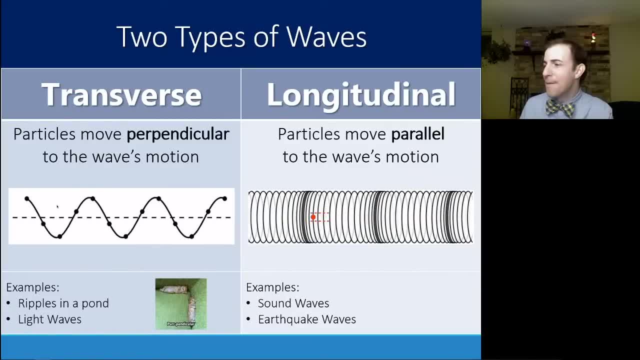 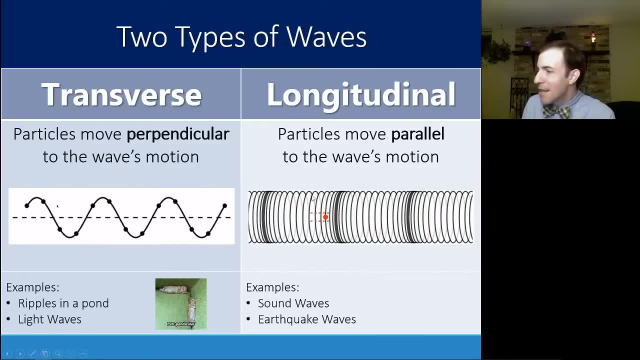 A good example of this is if you send, like a pulse, down a slinky, you can have areas of that slinky where the coils bunch up and areas where they spread out. But if you look at just one point in that slinky, that little red dot is vibrating back and forth left and right. 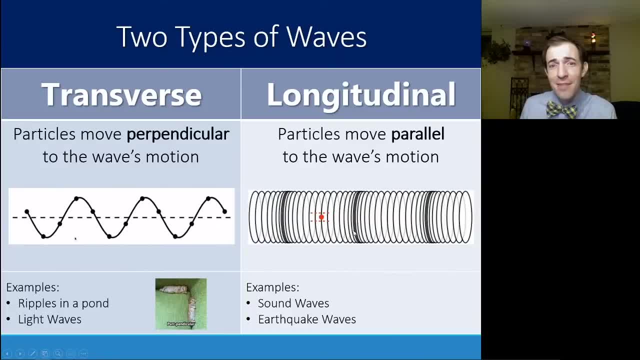 While that's, the wave is traveling left or to the right. here as well, These particles are moving parallel. These particles are moving parallel to the wave's motion. So examples of this- the key example that we'll talk about a lot- are sound waves. 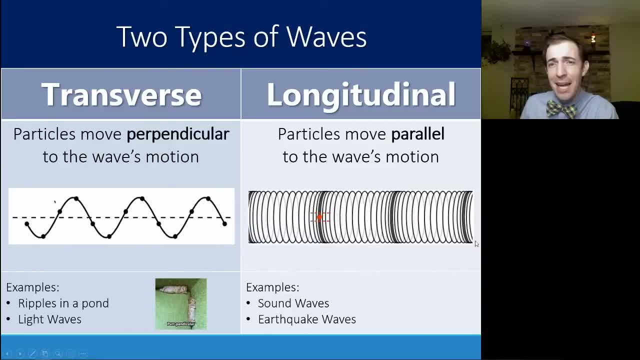 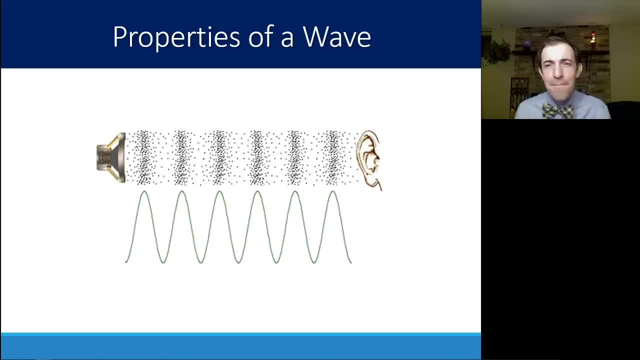 Earthquake waves can be both transverse or longitudinal depending on the type of wave. Now there are some different properties of these waves If we're going to use some vocab to define and talk about different parts of these. So we've got a transverse wave drawn here on the bottom. 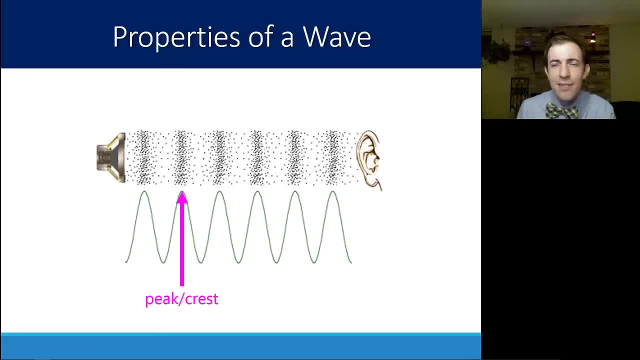 If we're looking at the highest point on that, we're going to call that a peak or crest- Either would be fine. The lowest point, we'll call that a peak, We're going to call that a trough. So if you hear me referring to a trough, or the peak, peak to peak, trough to trough, that's what I'm referring to there. 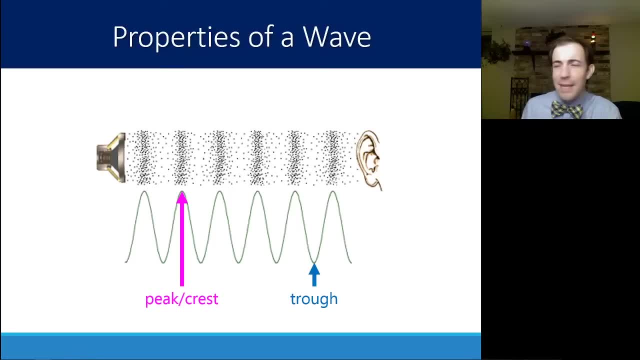 In a longitudinal wave it's a little trickier to draw. Here it's drawn out just air molecules being bunched together. So we have air molecules that have a high pressure. We're going to call that a compression That's analogous to the peak or the crest, the high amplitude here. 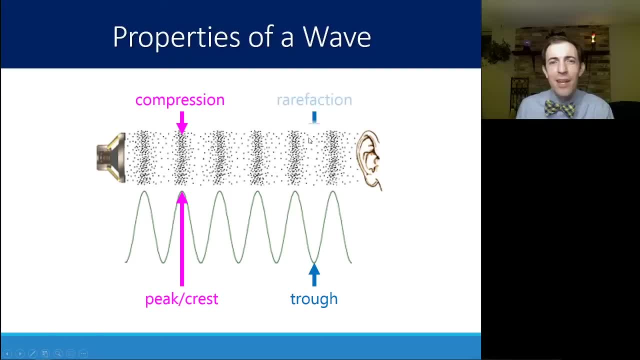 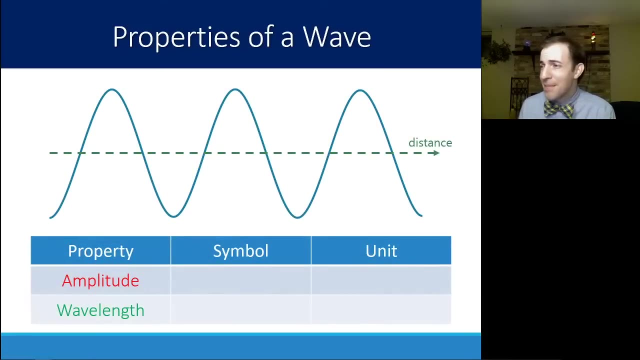 If we have a low pressure where the air molecules are spread out, We're going to call that a rarefaction. So compression, rarefaction are the same as a peak crest or trough in terms of longitudinal versus transverse, And some other properties that we can define just by looking at a picture of the wave are amplitude and wavelength. 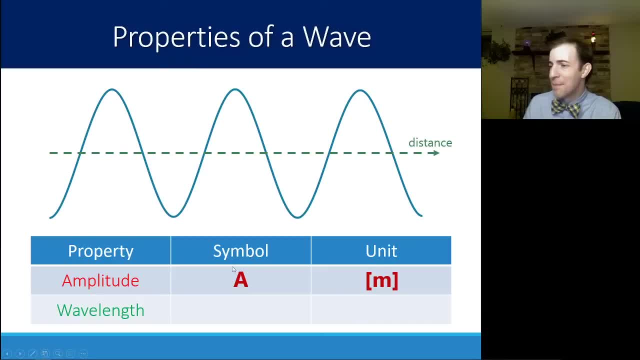 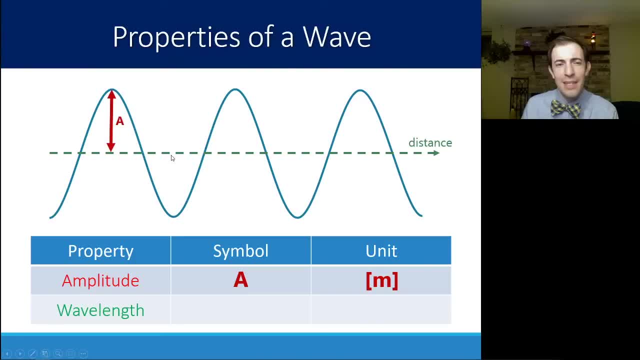 And that is measured from the high point here to the midpoint. That's our equilibrium point. that's the amplitude. You can also measure that. the equilibrium to the trough, That would also be the amplitude. It's the same thing. It's the same on the top and the bottom. 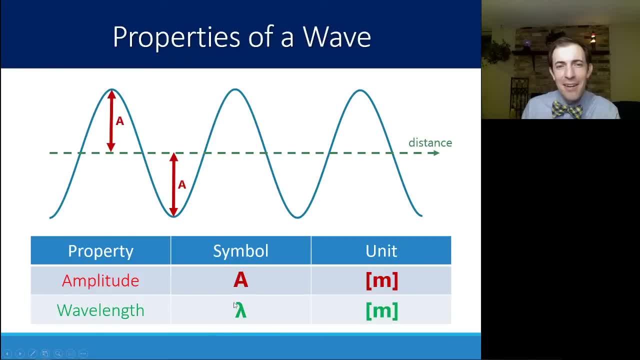 Wavelength is going to be measured using this Greek letter that kind of looks like a wishbone upside down. It is known as the Greek letter lambda, So this is a lambda here. that is also a length, so it's measured in meters. lambda wavelength is measured. 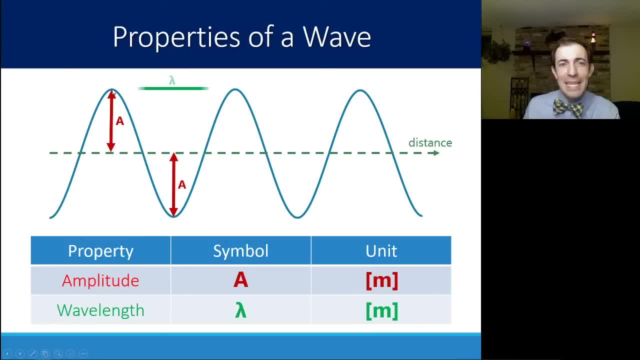 from two identical parts of a wave. so we go from peak to peak, or we can go from trough to trough, or, if you start in the midpoint, you just need to make sure that a full wave has gone by, going up to the peak and down to the trough, so we have a 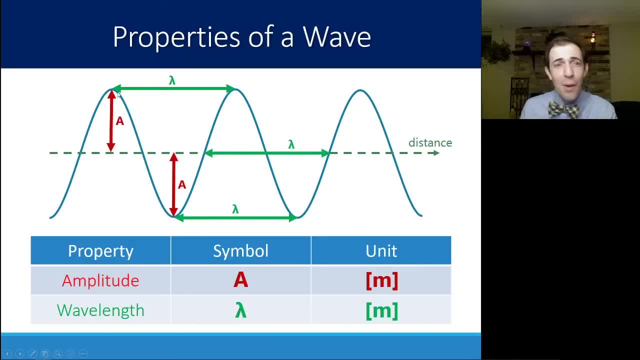 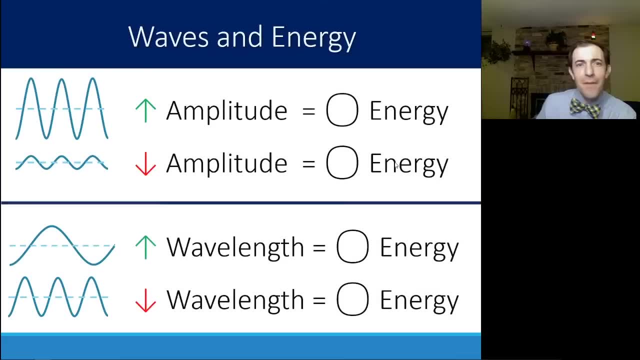 wavelength. here these are all symmetrical as well, so all of these wavelengths are equal to each other, no matter how we draw them all right, waves carry energy. the higher the amplitude, the higher the energy that is carrying. the lower the amplitude, the lower the energy. and just looking at 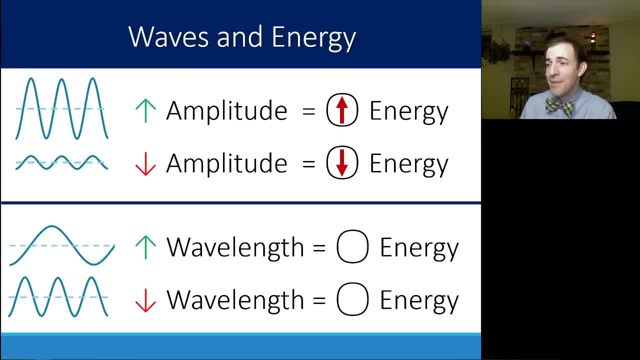 those pictures you can kind of get a sense of that. in terms of sound, a high amplitude would be a very loud sound. in terms of light, a high amplitude would be a very bright light. a wavelength also results in different energies. you can kind of imagine what that would be looking at. 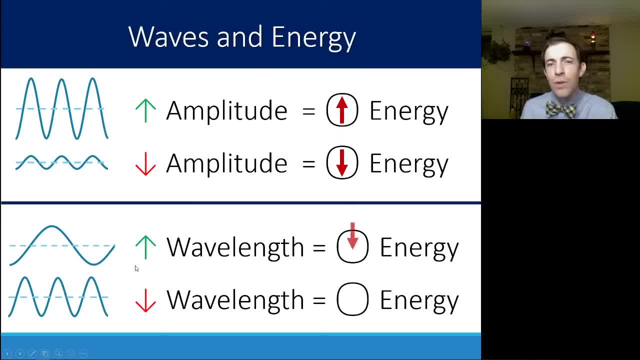 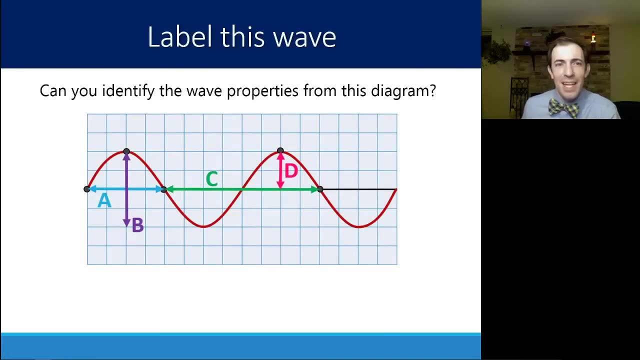 these pictures as well. these are really long wavelengths is a lower energy wave and a higher. higher wavelength you have more waves per second. presumably we'll have a higher energy. so a low wavelength is a high energy. a high wavelength is a low energy, all right. so looking at this diagram, 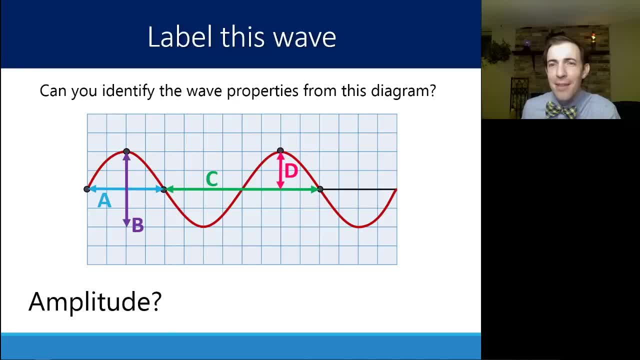 can you identify the wave properties first? i would like you to identify which of these is the amplitude of the wave. of course the amplitude here is not the highest point to the lowest point. the amplitude is how far away it is from that equilibrium. so our amplitude is actually point d or the. 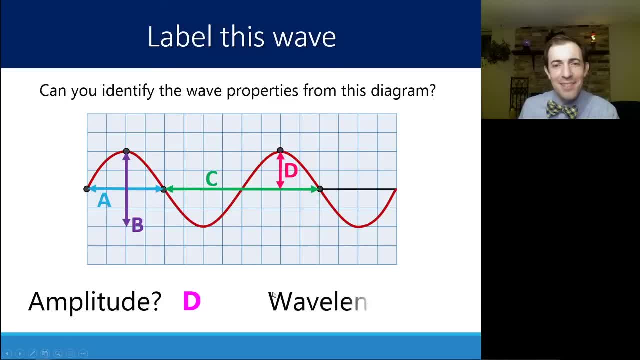 the length represented by the arrow d. next, which of these a, b, c or d represent the wavelength of this wave? wavelength is between two identical parts of the wave, where a full complete cycle has a complete cycle of a wave length and a complete cycle of a wave length. 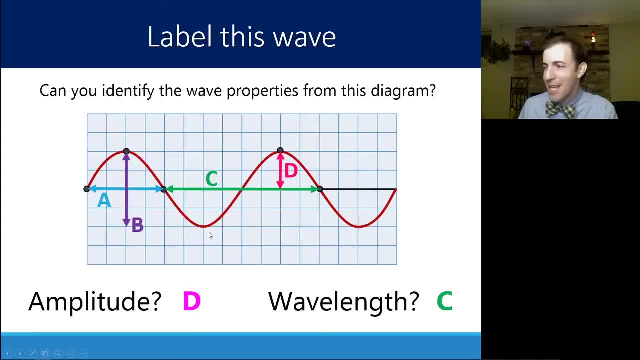 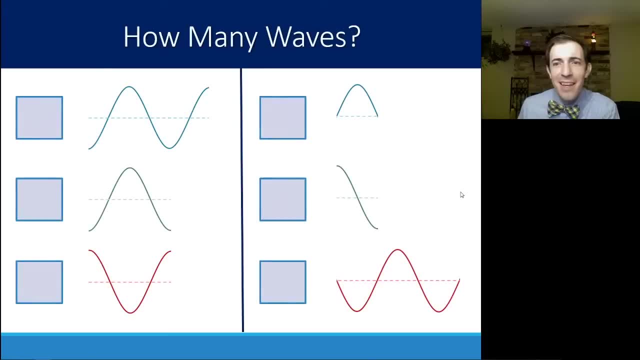 occurred between uh and that is c, where it goes down to the trough, back to the peak and then back to its original position. next, you need to know how to count the number of waves. just looking at a picture and there's a variety of different ways that the wave might be drawn out. uh, here to start. 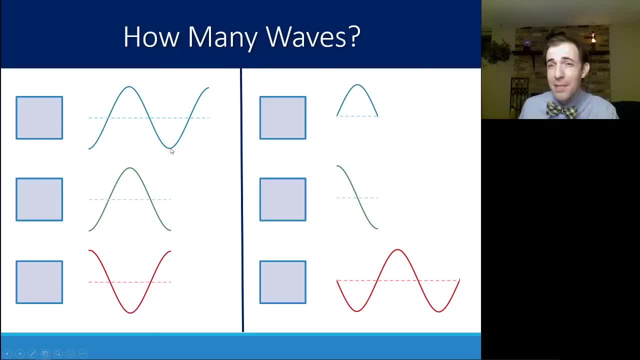 with. we start at the trough, we go to the peak and back to the trough. that's one complete wave and then back to the peak. that's another half of a wave. so we would say that that is one and a half waves. uh, here we've got. 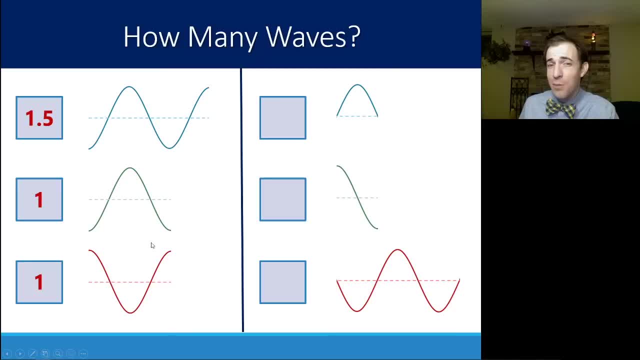 trough to trough, that's one complete wave. peak to peak is one complete wave. here we start in the middle, we go to the peak but we don't go all the way down to the trough. so we only have done half of that wave. so we call that 0.5 um. next, if we start at the peak and go all the way down to the 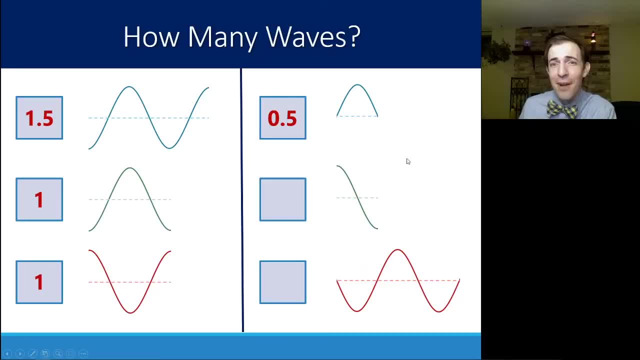 trough. we'd have to go all the way back to the peak for that to be one complete wave. so that's also just half a wave. uh, looking at this last one, how many waves are there in this final example? we start out in the middle, we go to the trough, to the peak and back. that is one complete wave. 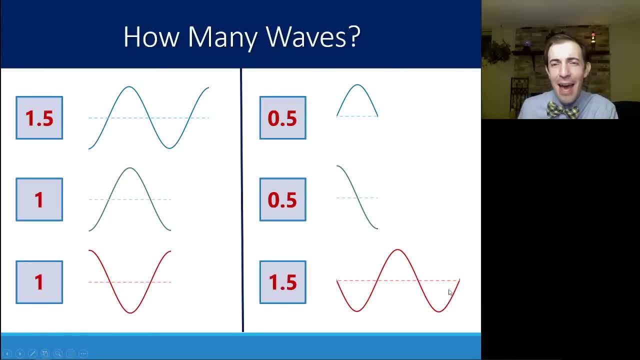 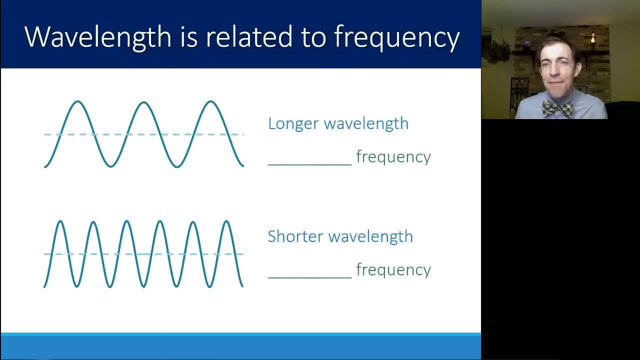 and then we have another half a wave. that gives us one and a half waves. so this idea of wavelength and frequency are often very much related to each other, because most waves of a given type will travel at the same speed. so if you have a longer wavelength, you are going to encounter less waves per second. 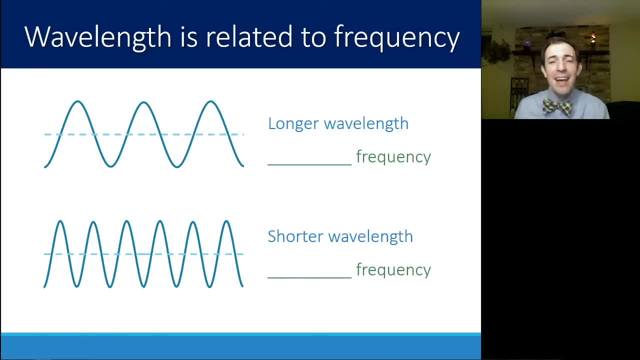 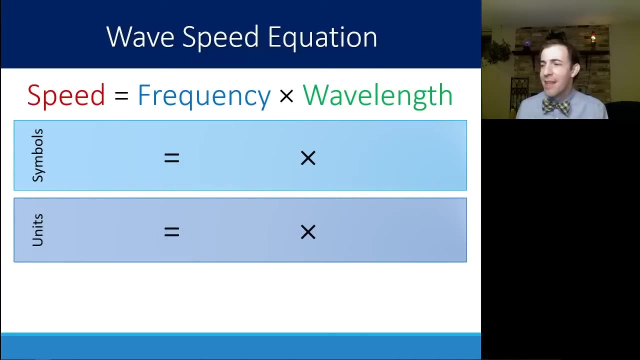 just because it takes more time for a long wave to pass. that would result in a lower frequency. if you have a shorter wavelength, you'll have more waves per second. waves per second is a higher frequency in this case. so that leads us to a mathematical relationship that can relate speed of a wave, frequency and the wavelength, and that speed is represented. 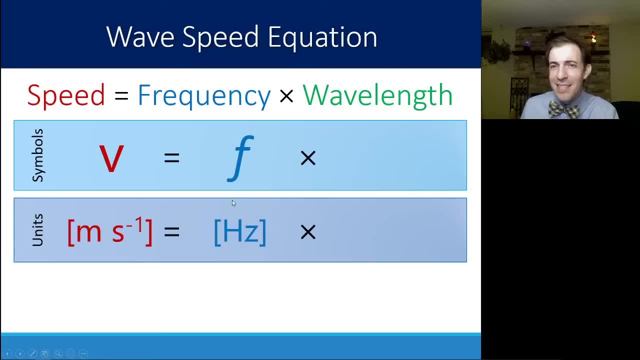 typically with a lowercase v in meters per second. frequency is that italic f? uh in hertz and wavelength is lambda in meters. so we have v is equal to f times lambda frequency times wavelength. looking at these units, uh, it doesn't look like the units work. hertz times meters is meters per second. well, you have to know that hertz is actually a derived unit. 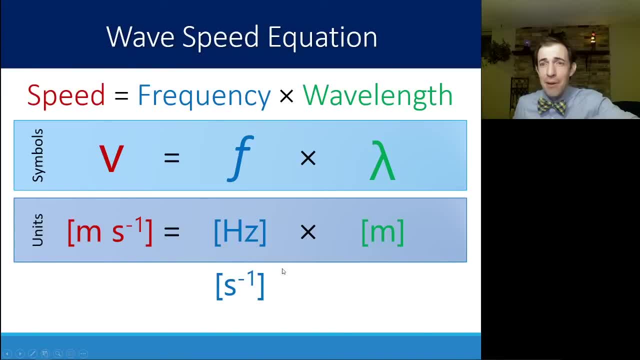 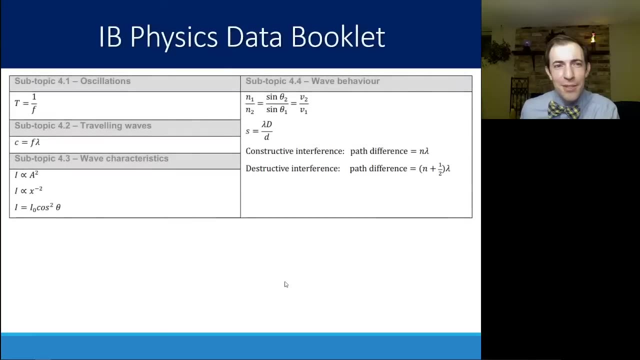 one over seconds. so it's a number of waves, which is just a number, a perfect number, no unit divided by seconds. so one over seconds is hertz, which means that one over over seconds times meters is meters over seconds, meters per second. so we can use this equation. 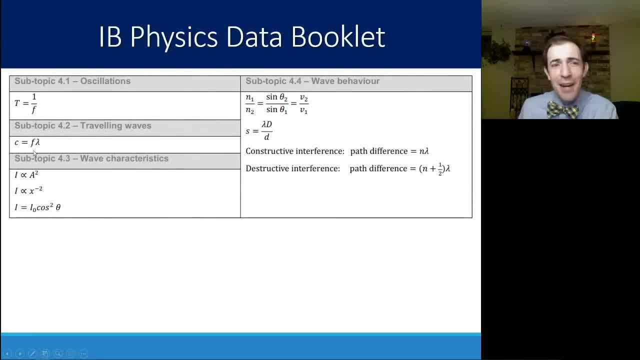 um, because it shows up in your ib physics data booklet. it shows up here in subtopic 4.2. now i want to point out something here. c is representing the velocity. that's technically actually the, the speed of light, and that's how you represent the velocity of light. uh, but the 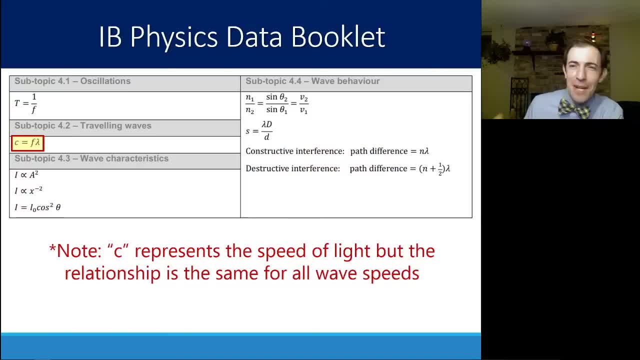 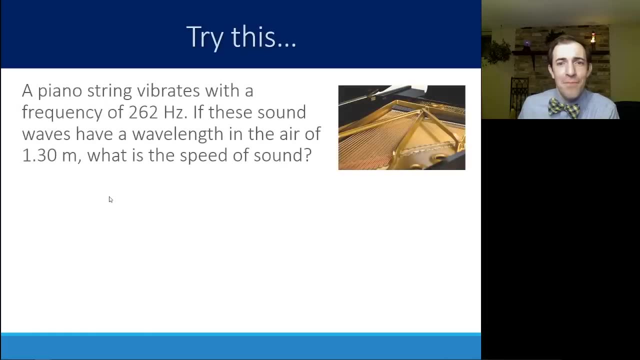 same relationship holds true for all wave speeds. uh, whether you're talking about sound or a water wave, uh, it's just. for whatever reason, the, the equation that's given to you is specifically for light, but you can substitute any velocity in for c, so let's try an example here: a piano string. 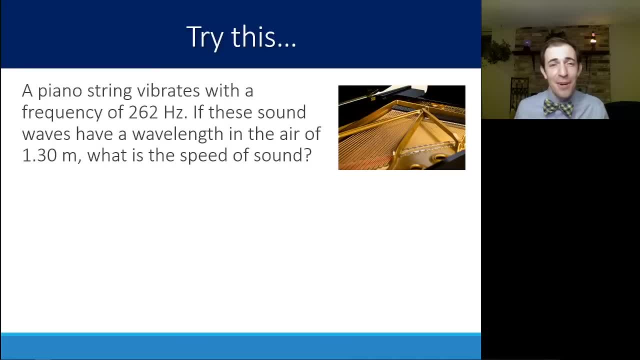 uh vibrates with a frequency of 262 hertz. uh, which means 262 vibrations every second. if these sound waves have a wavelength in the air of 1.3 meters, what is the speed of sound? so these are my givens um. i know that my speed is just frequency times, wavelength um, so so from that i can. 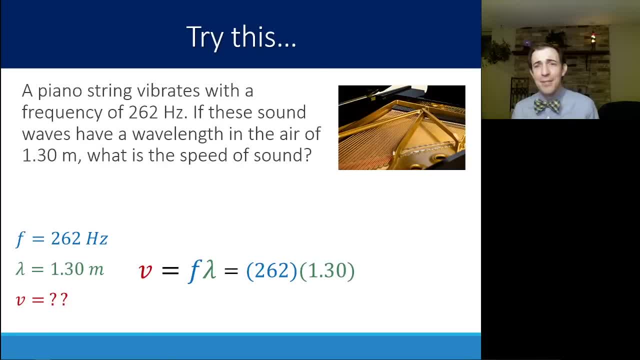 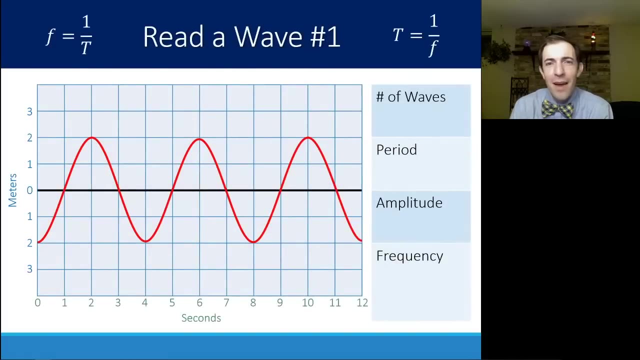 calculate what the speed of sound should be. 262 times 1.3, the wavelength results in about 340 meters per second. that's roughly the speed of sound in air, which we'll see a little bit in a future lesson. i should be able to read the speed of sound in the air, but i don't know how to do that. 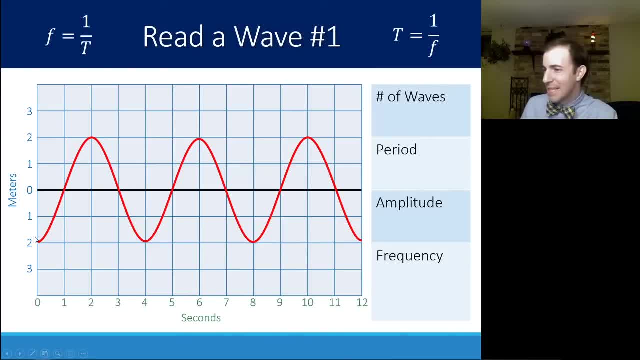 i don't know how to read the speed of sound in the air, but i don't know how to do that. i can read a wave as well from any picture. so if i see this, i've got three complete waves um the the x-axis. here is time, so i can read out the period just by looking at two identical parts. 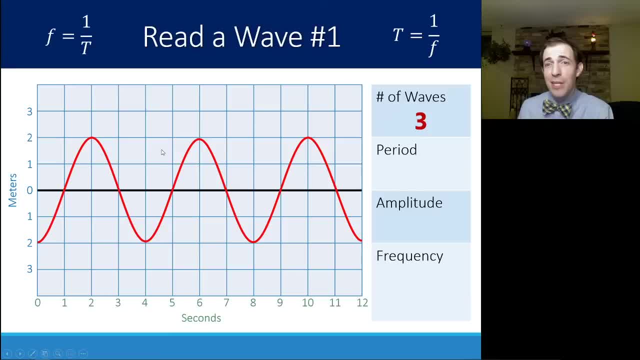 of the wave, peak to peak or trough to trough. um, the separation is always four seconds, so it takes four seconds for a complete period of the wave. the amplitude here is the distance from my center point. so that is two and not four, and you're not going from trough to peak. 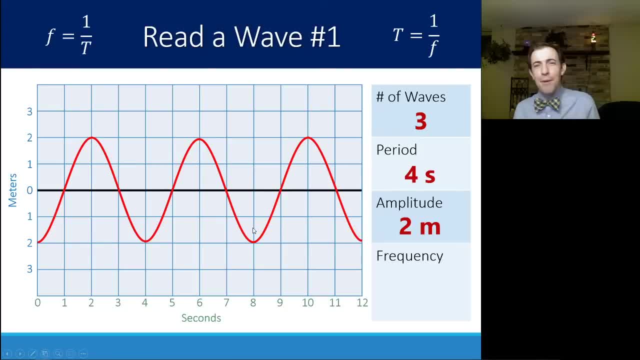 going from peak to the equilibrium and then frequency can't be read directly from the wave, but if you know the period you can find the frequency. the frequency is how many waves per second? well, it takes four seconds for one wave, so the frequency is just one divided by four, or 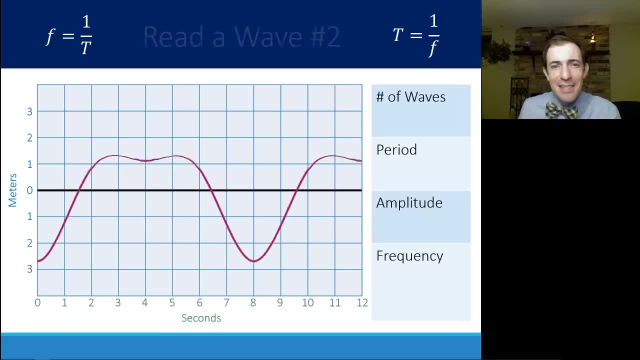 point two: five hertz. i can do this in another example as well. um, here, uh, there are: there's one complete wave and another half, so that's one and a half waves. the period is the time from trough to trough, that's eight seconds. the amplitude in this case is three. um, go ahead and figure out what the 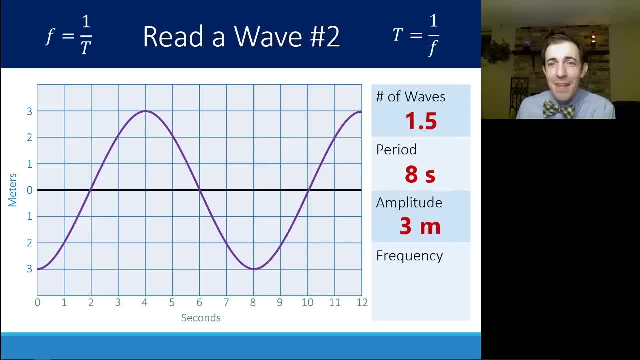 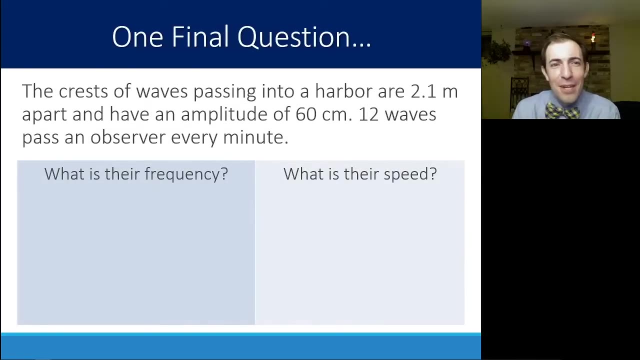 frequency should be for this wave. if you know the period, the period is eight seconds. the frequency is just one divided by the period. so point one, two, five hertz: you experience an eighth of a wave every second. all right, one final question for you before we are done with this lesson. 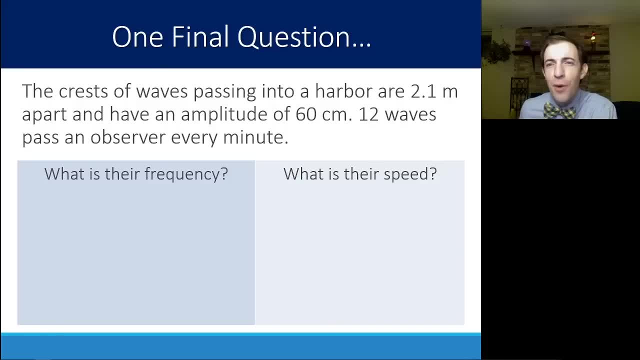 the way. the crest of waves passing into a harbor are 2.1 meters apart and have an amplitude of 60 centimeters. 12 waves pass by an observer every minute. i would like to know the frequency and i'd like to know the speed. so first go ahead and figure out what is the frequency, if you 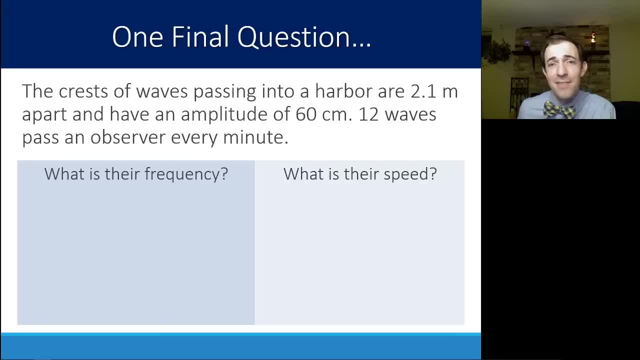 have 12 waves every minute. what's the frequency in hertz? well, hertz is just number of waves per second. so, um, i know that there are 12 waves per minute and then there are 60 seconds in one minute. i can use dimensional analysis and cross off minutes and i get waves per second. 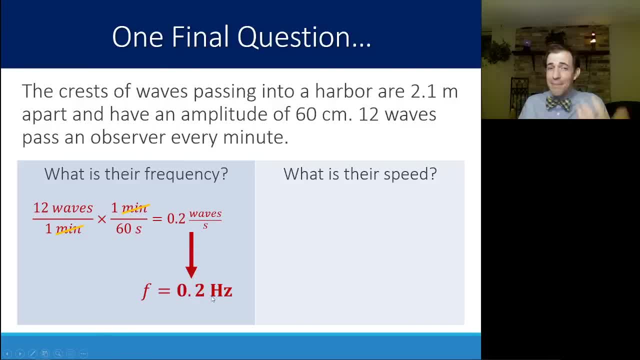 12 divided by 60 is 0.2 waves per second. that's the same thing as saying 0.2 hertz. if i want to find the speed, then i now know the frequency and i know the wavelength. the wavelength in this case is not 60 centimeters. that's the amplitude, the wavelength is the. 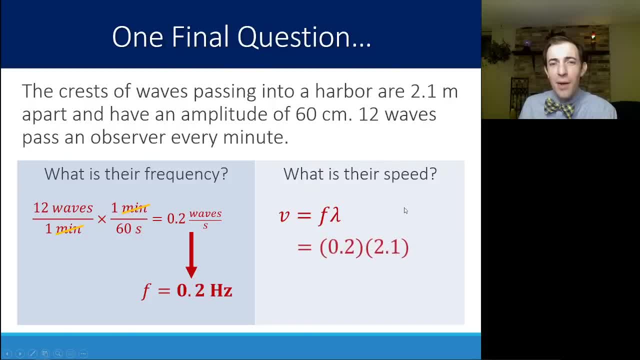 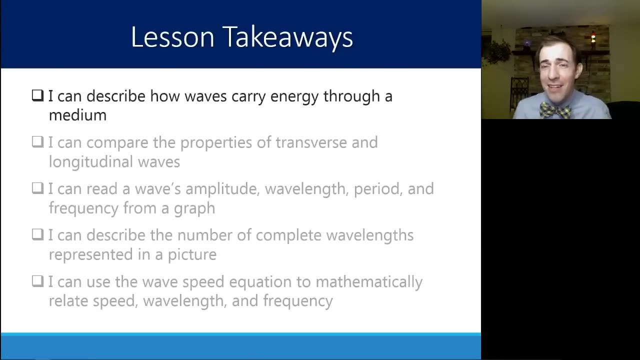 distance between crests. that's 2.1. so i got 0.2 hertz times 2.1 meters will give me 4.2 meters per second for the speed of that wave. in this lesson you should be able to describe how waves carry energy through a medium and describe 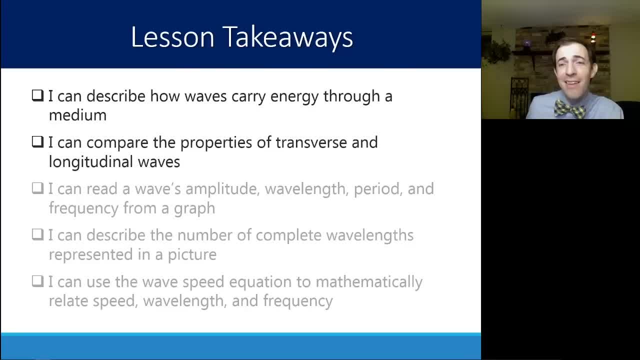 what that medium is and how it vibrates. you should be able to compare and contrast properties of transverse and longitudinal, which one is perpendicular, which one is parallel. you should be able to read a wave's amplitude, wavelength, period, frequency, as well as crest trough compression. describe the number of complete wavelengths from a picture and then use the wave speed. 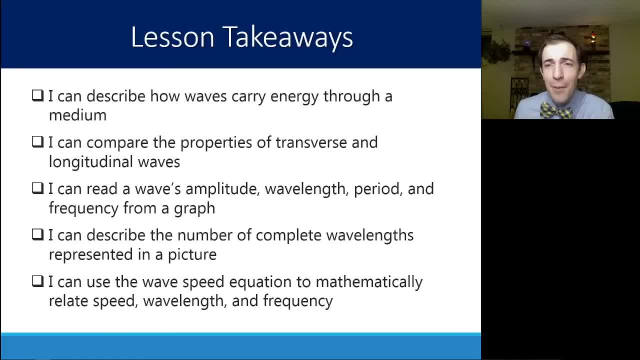 equation to calculate for an unknown, whether it's speed, wavelength or velocity.